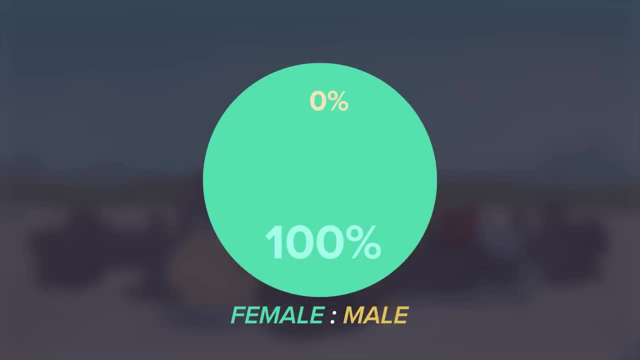 and don't contribute anything to the next generation. Yet even though it would be a lot more efficient to have just a few males and a bunch of females, roughly equal numbers of each sex are born every season. We see this in almost every animal species on Earth. 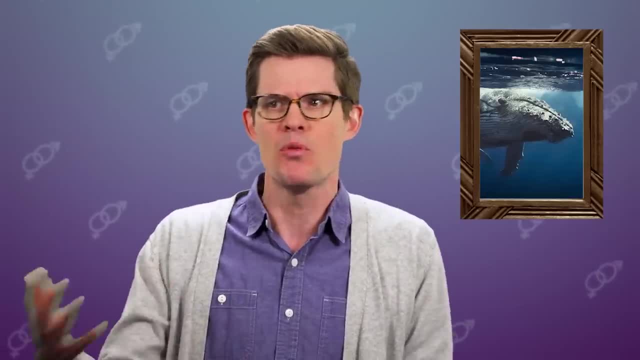 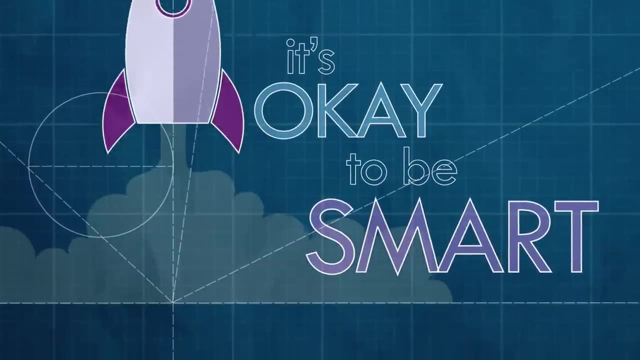 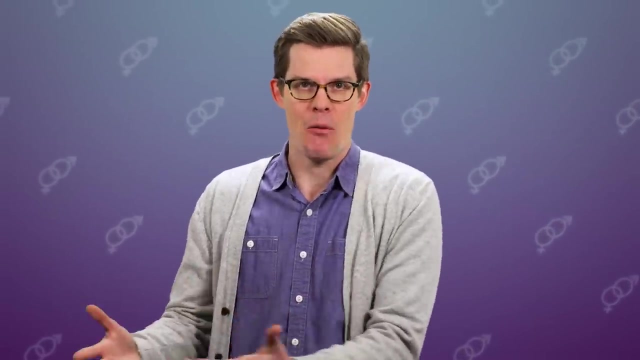 Why do most animals, from eagles to armadillos, to blue whales to us, make equal numbers of males and females? The equal ratio of sexes is so common in nature. most people never wonder why it is that way, And it's worth pausing here. 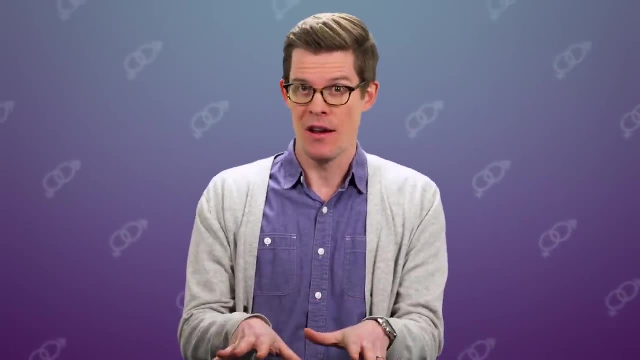 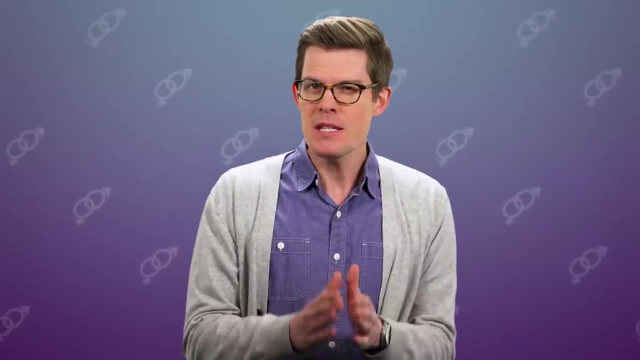 for a second to make clear: we're talking about biological sex, not gender. You probably learned that when male and female chromosomes shuffle and combine, there's a 50% probability of either sex. But this just tells us how it is, not why it is this way rather than. 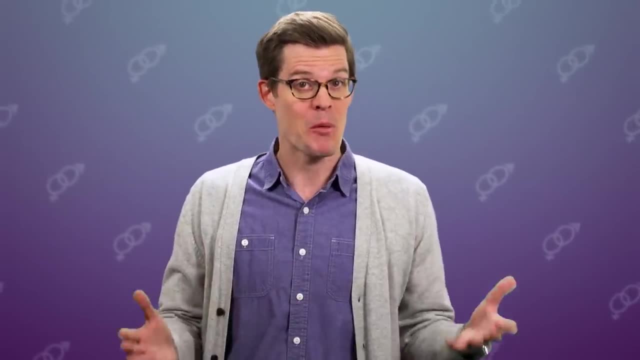 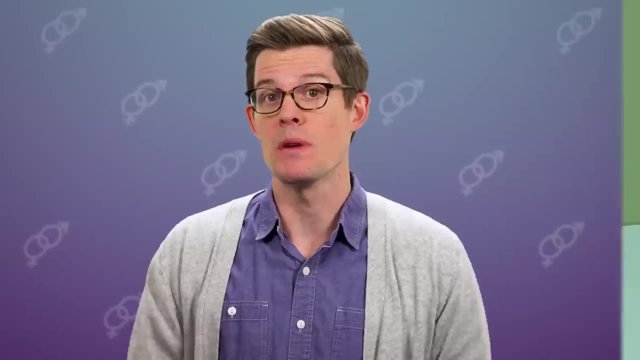 some other way, And in biology that's really what we want to know. If getting your genes from one generation to the next is the whole point of evolution, then you'd think the best strategy would be to put a lot of eggs into the female basket. 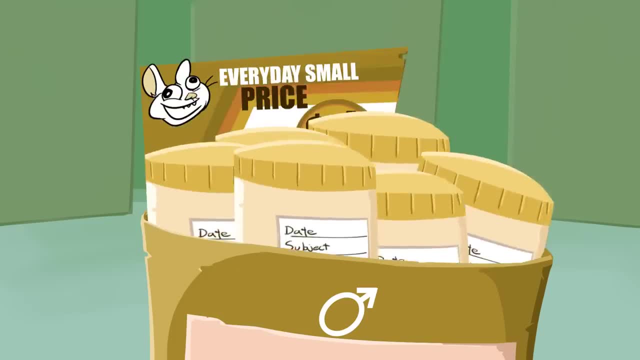 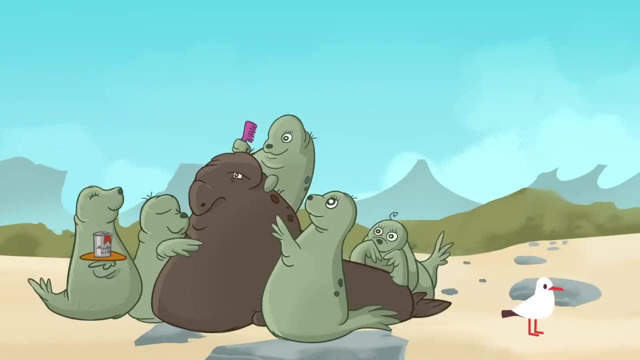 Worms are really cheap to produce, so males make a lot of them, And animal males typically don't do most of the childcare, So you get a situation in which you only need a few males to keep a population churning along. This seems like the ideal situation, not just for 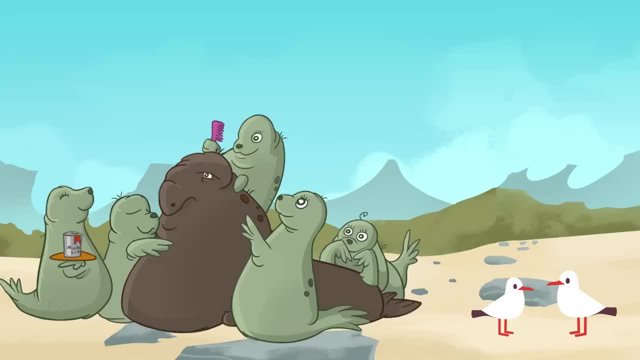 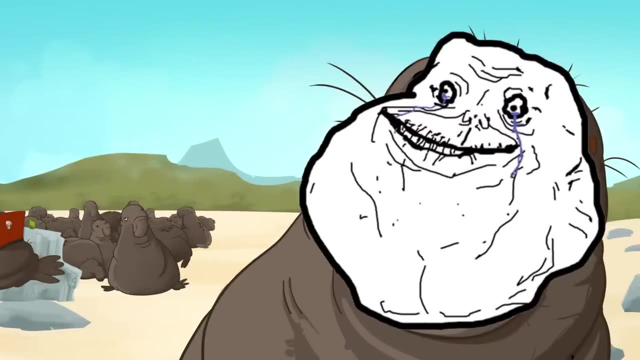 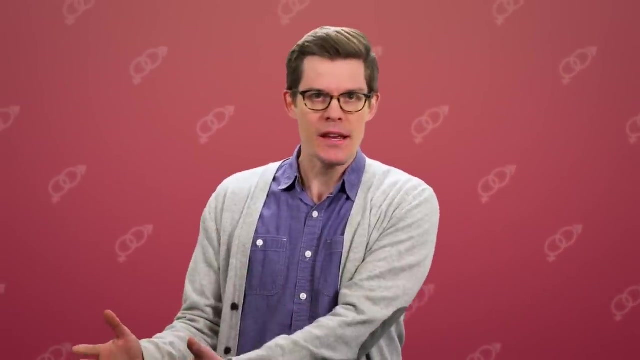 elephant seals, but for many animal species Yet. elephant seals produce both sexes in equal numbers, and the result is a whole lot of mooching mateless males. As far as evolutionary strategies go, this one seems like a lot of fun. It's not survival of the moochiest, it's survival of the fittest Fittest in biology. 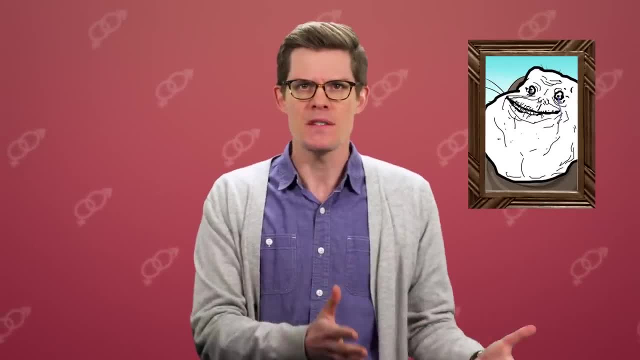 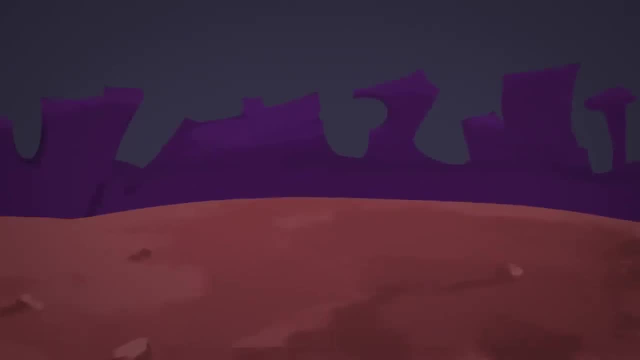 means makes the most offspring, And 96% of elephant seal males get a big zero for fitness. That's totally bonkers. So how can we explain it? Let's start with a hypothetical population of purple people-eaters in which, out of every 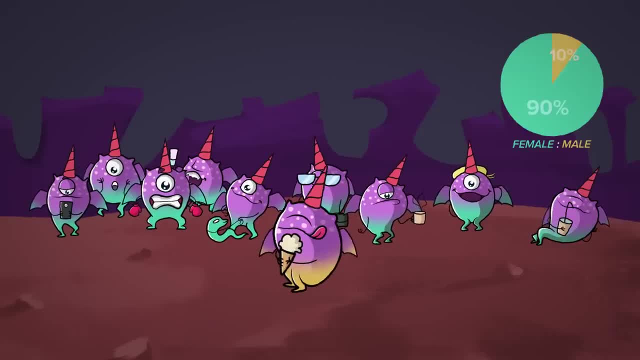 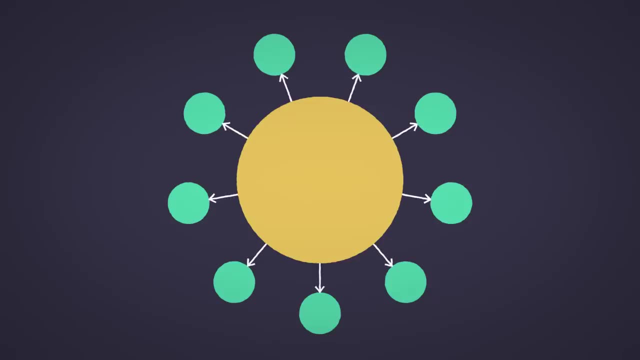 ten purple people-eating babies born. nine are female and one is male. When it comes to making adorable people-eating babies, every male will get to mate about as often as every female. If every mating results in two new purple people-eaters, then 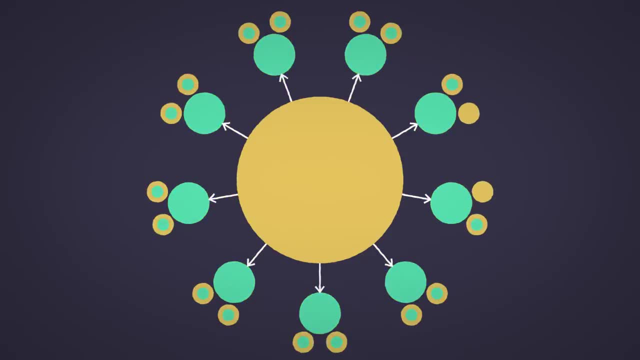 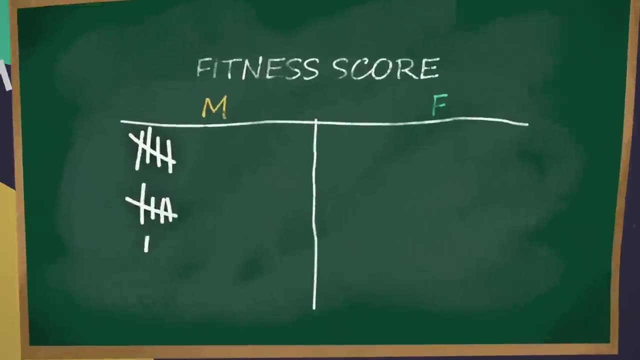 in the next generation. each male's genes are carried on by 18 offspring, but each female on average gets their genes into just two. When we count up the fitness score, every male in this population has nine times the fitness of every female. 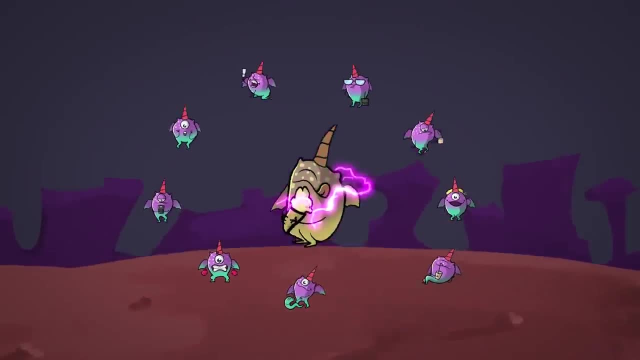 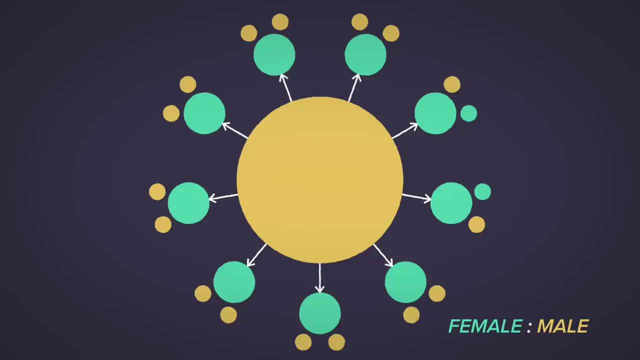 If, through the random chance of evolution, one muncher manages to change in a way that it produces, say, nine male kids for every female kid, those offspring would have to have a huge advantage in this population. With this genetic change, one of these new 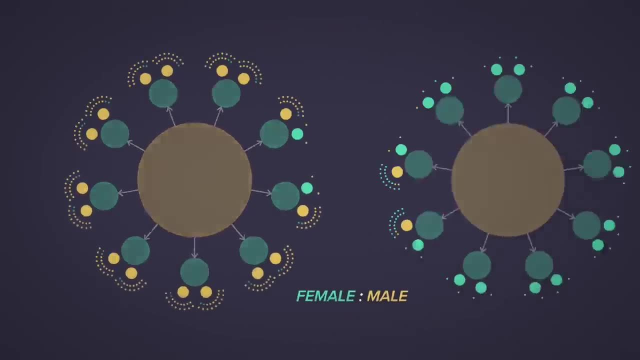 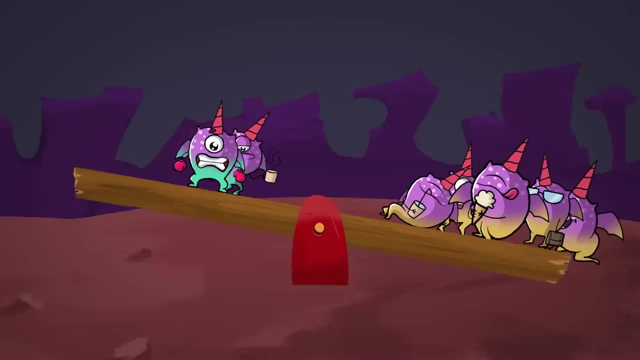 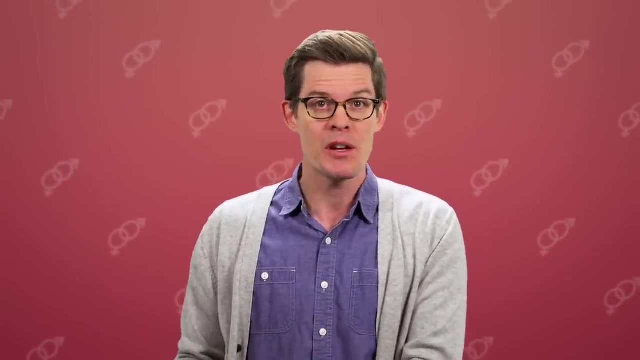 males would produce roughly four and a half times more grandchildren than a male. without the change. This new mutation will spread like gangbusters and in a few generations you'd have more males than females in the whole purple, people-eater population. But at this point the mutation causing 90% male offspring would no longer be an advantage. The environment has changed and now females are the rarer sex. Now, if we're talking about a male offspring, we're talking about a female offspring. If any parent with a mutation that results in extra female offspring would be favored, then that mutation would spread until the sex ratio moves back towards more females. Repeat this. 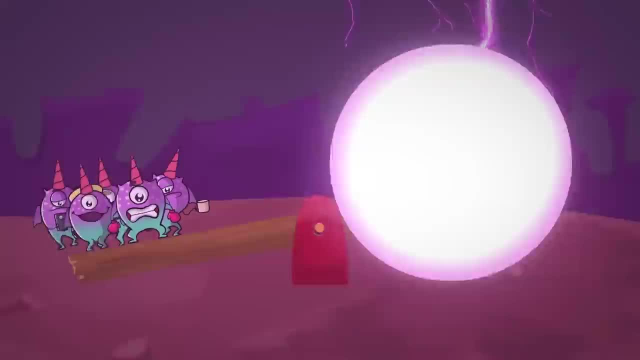 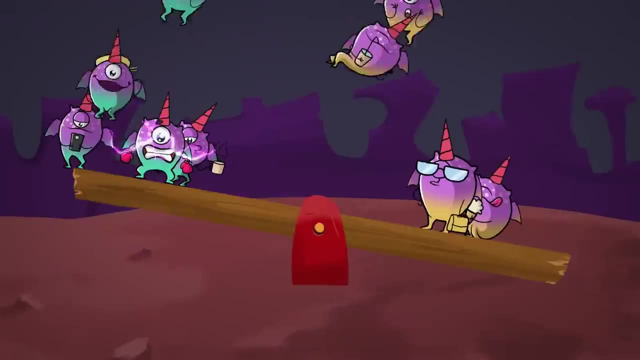 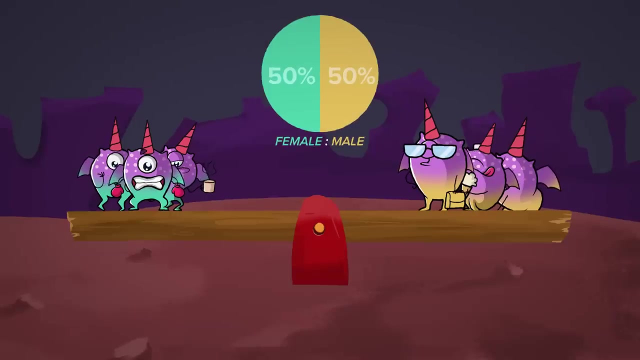 whole process and we move back towards more males, then more females, then more males. The population would be in a constant seesaw towards one sex or the other until finally a mutation arises that results in an equal ratio of offspring, That magic 50-50 sex ratio. 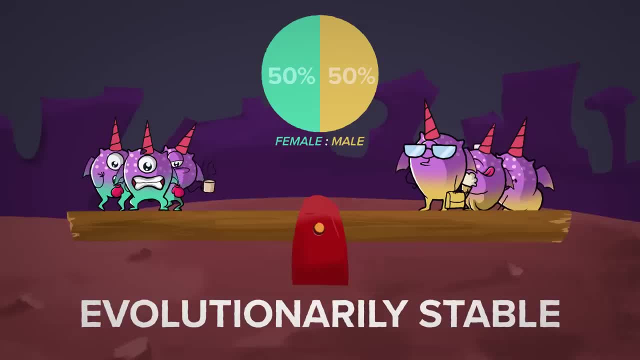 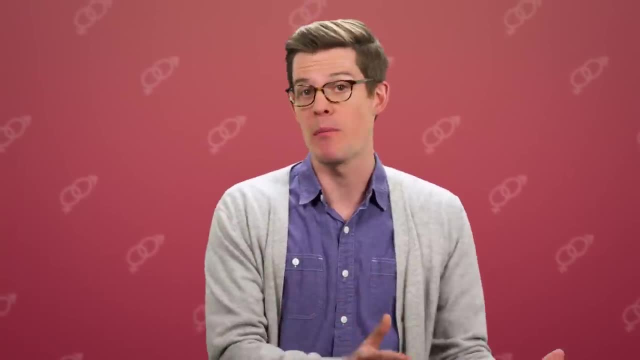 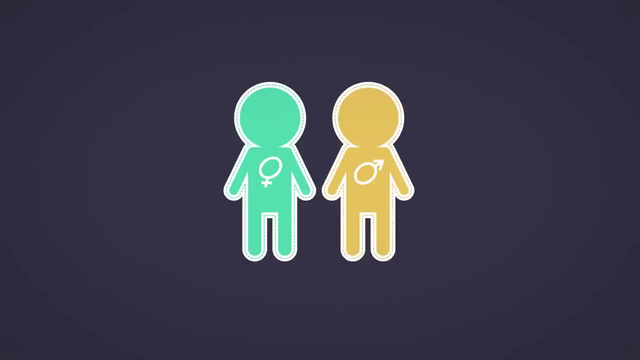 is the only one that is evolutionarily stable, And that right there is why we see it again and again, and again. Of course, the 50-50 ratio isn't just about numbers of offspring. It's really about how much time and resources parents invest in offspring. We see 50-50 sex ratios whenever. 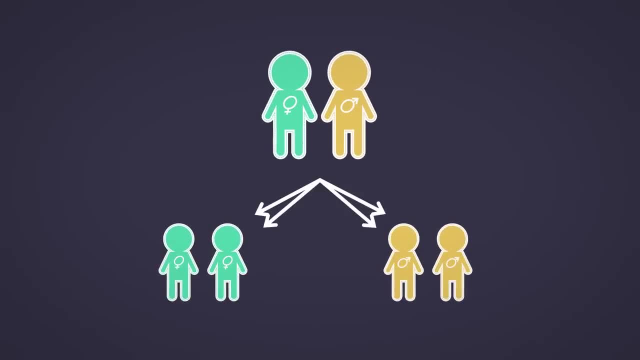 parents invest equally in their male and female children. If investment is unequal, like if females require twice the parental care of males, you'd expect to see twice as many males born than females- Sure, But if each male has less chance to pass on their genes, they cost half as much as females. so it evens out. Australian brushtail possum moms, for example, invest more resources in their daughters and those daughters live in the dens with their moms, So when these resources are scarce, they have more male offspring. Like everything in biology, there are lots of weird exceptions to this, But it's amazing.